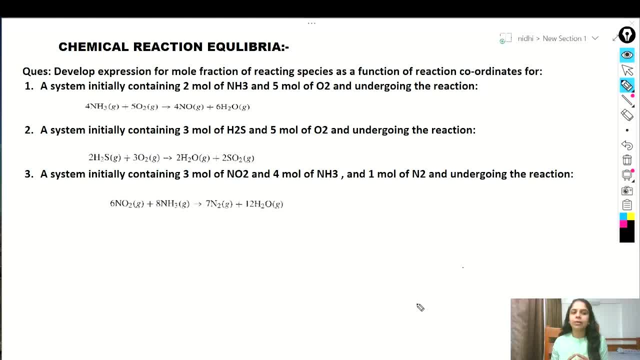 Hi everyone. so in our today's video we will solve some numerical problem based on reaction coordinate. So let's solve the problem: Develop expressions for mole fraction of reacting species as a function of reaction coordinates. for first, a system initially containing two mole of NH3 and five mole of oxygen and undergoing the reaction, and the reaction is given to us. 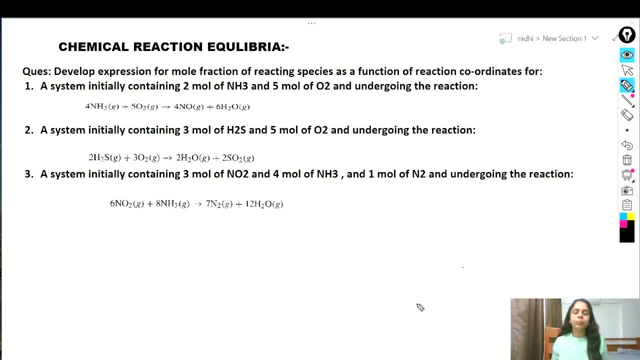 it is 4 NH3 plus 5 O2 gives 4 NO plus 6 H2O. and then the second question is a second part of this question is a system initially containing three mole of H2S, hydrogen sulfide and five mole of oxygen and undergoing the reaction, and similarly, third part is also given to us. So 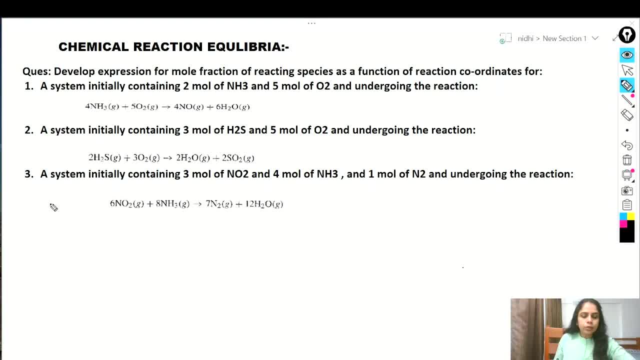 let's start the first part. Okay, so first part, first reaction is a system initially containing two mole of H2O and five mole of oxygen and undergoing the reaction. and similarly, third part is also given to us, So let's start the first part. Okay, so first part, first reaction is a system. 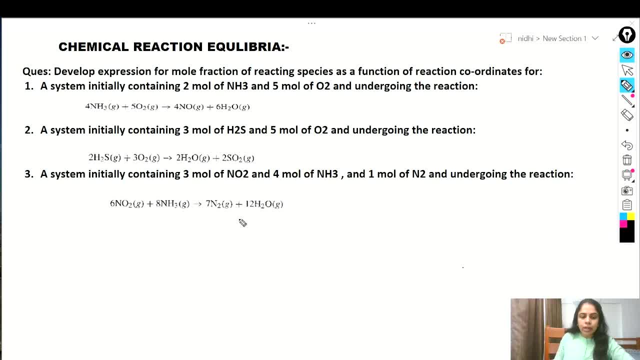 initially containing two mole of NH3 and five mole of H2O and undergoing the reaction and incoming two mole of NH3 and five mole of H2O, and undergoing the reaction and accompanying the reaction. and then we know that the reaction coordinate formula which we have derived in our previous video. So 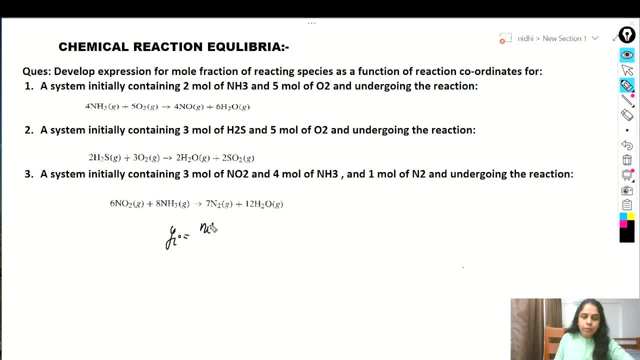 it is. yi is equals to initial number of mole upon total number of mole, which is equals to ni0 plus mui epsilon upon no plus mu epsilon. okay, so first total number of moles are which is given to us, so total number of moles. 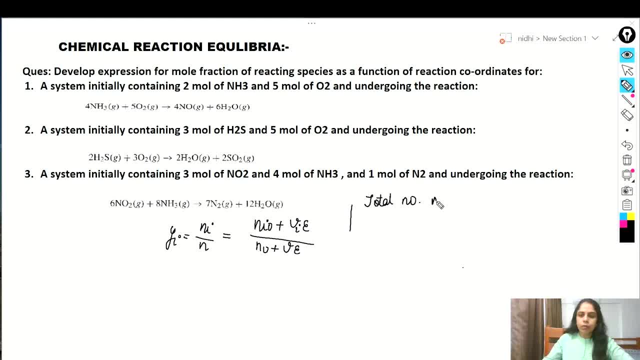 for the first reaction. total number of moles for the first part. right, this is for the first part. so, uh, how much, two mole plus five moles, so seven. so total number of moles and o is seven moles right now. species: how many species are there? so we just i, uh, we know that i is for species. 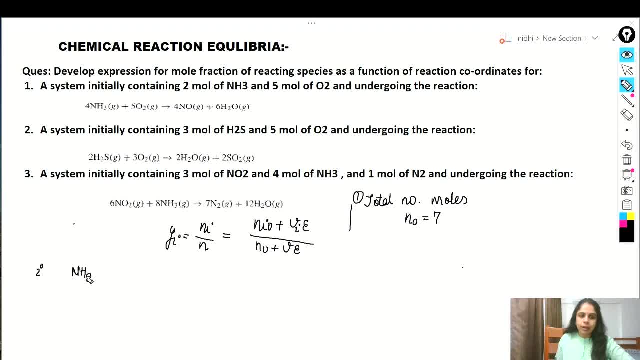 okay, so just write down. so reactants, ammonia, then oxygen and products are n, o and h2o right now their stoichiometric stoichiometric coefficient. so, uh, ammonia stoichiometric coefficient is four. so we know that for the reactant it must be negative and oxygen, the stoichiometric coefficient is five. so minus five. this is because these two 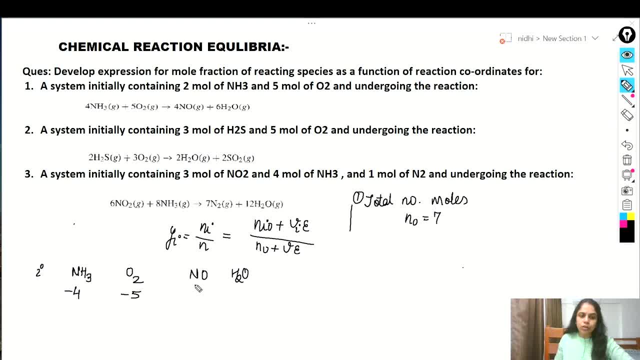 are the reactants and products are n, o and h2o. so stoichiometric coefficient for the n? o is four and for uh h2 it is six. fine, now here we can write like this: so total number of uh, stoichiometric coefficient of uh, this is for: 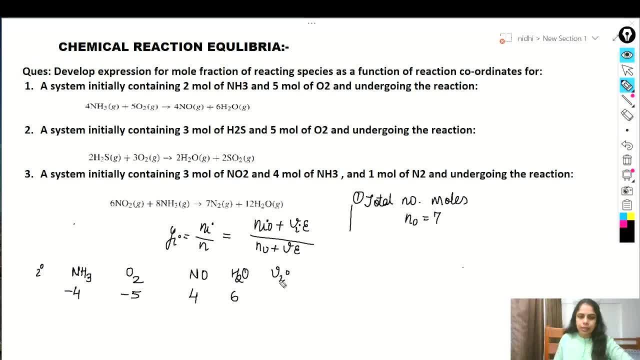 the individual and total of uh. this is for the individual and total of uh. this is for the individual and total for the total reaction. so when you add this, you will get minus four, minus five, four, four, cancel. so it will come one. fine, so new. the value of new is new. this is the new. okay, not new, i it. 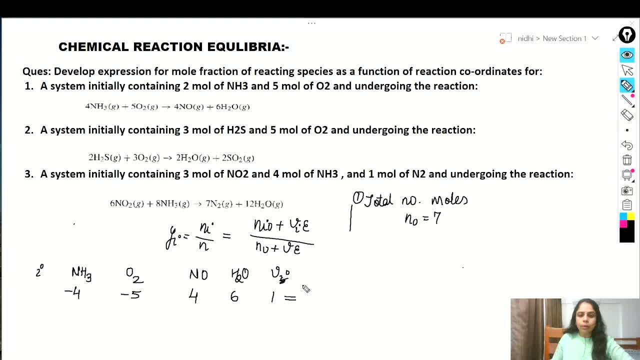 is new, okay. so new means it's a total number of uh stoichiometric coefficient, coefficient for the reaction. now let's start the mole fraction. so first we need to find out the mole fraction for ammonia. so y, nh3. so just put all the values in this uh given formula, so ni o ammonia, uh the given. 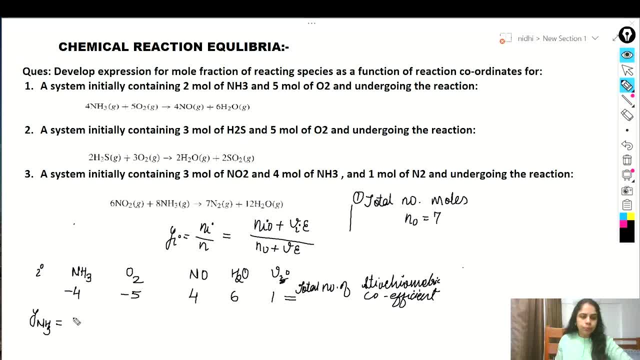 initial number of ammonia is two mole, so two. this is the initial number of ammonia. so the initial nio is for the initial number of mole of individual species or individual component. so we are writing this, we are finding the mole fraction for the individual individual component right, and we are writing the expression of mole fraction in terms of. 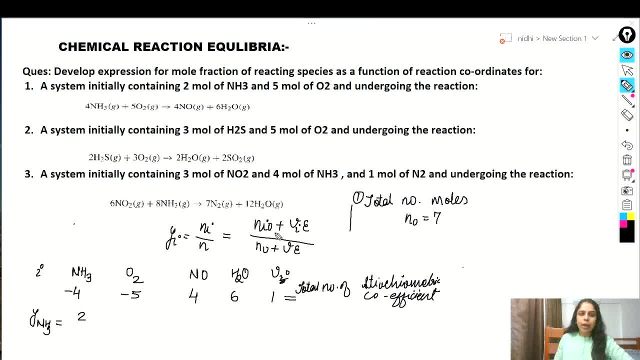 epsilon or reaction coordinate. fine, so nio it is, given the initial number of mole of ammonia is 2. fine then, plus nu i, epsilon, so nu i. that means the stoichiometric coefficient of individual component, so which is minus 4, so here plus minus 4, and epsilon is remain same. 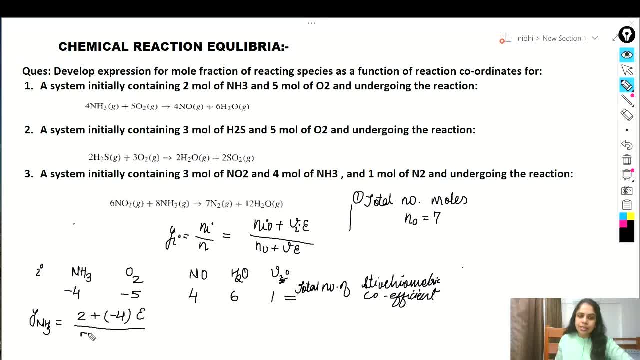 then n total number of moles are 7 plus total stoichiometric coefficient of the reaction is 1 epsilon. so this will be equal to 2 minus 4 epsilon. epsilon upon 7 plus epsilon right, this is the first. now find out n mole fraction of: 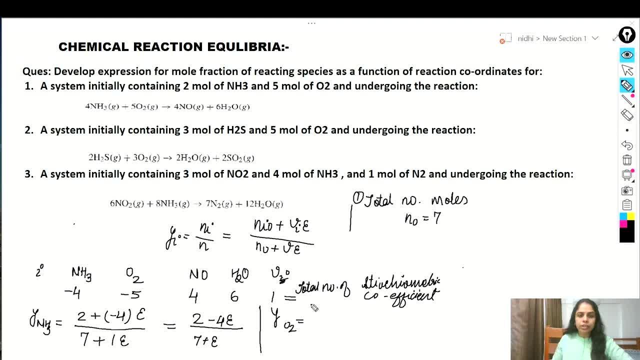 O2, oxygen. so this will be equal to initial number of moles, for the oxygen is 5. find a stoichiometric coefficient is also my 5. so minus 5 epsilon upon. and the denominator part is remain same for all the, all the species right now. third is Y and O. so initial number of moles. 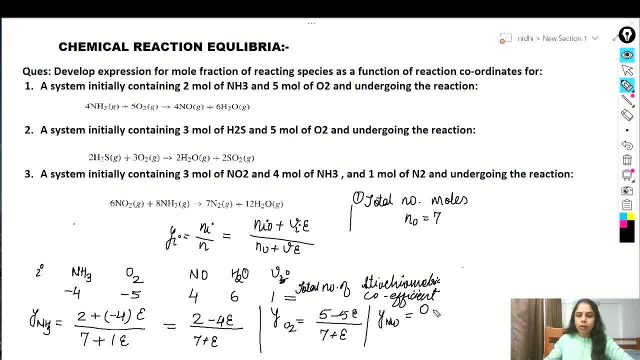 are not given, so that will we need to consider as 0 plus stoichiometric coefficient for the NO is 4 epsilon upon denominator is remain same for this also, so this will be equal to 4 epsilon upon 7 plus epsilon. now the next last part is: 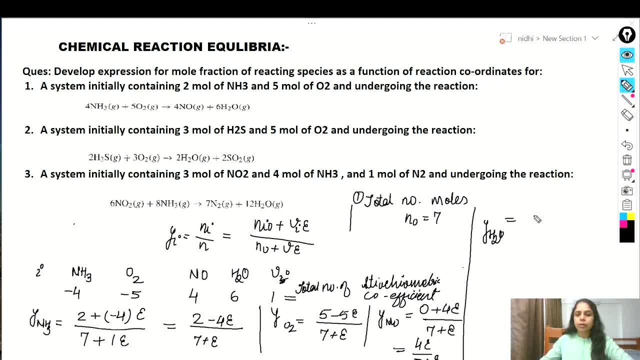 Y and O. so initial number of moles are not given, so that we need to consider as 0 plus H2O. so initial number of moles are not given, so that will be equal to 0. plus is stoichiometric coefficient for the H2O is 6 epsilon upon 7 plus epsilon, so that will be. 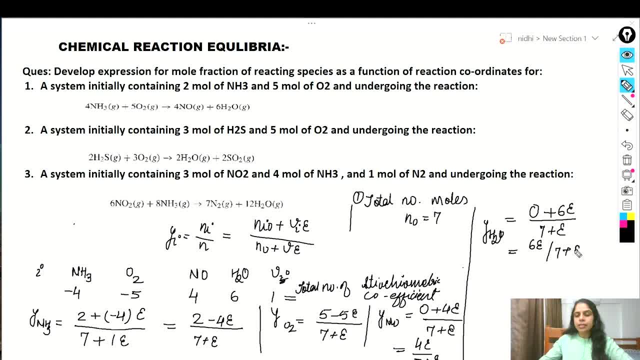 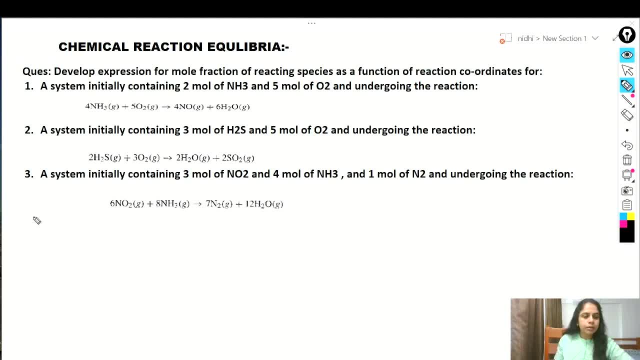 equal to 6 epsilon upon 7 plus epsilon. so these are the four expressions for the first reaction. for the second part. now for the second part, again, we write the number of components for the first reaction. so we write the number of components for the second part. 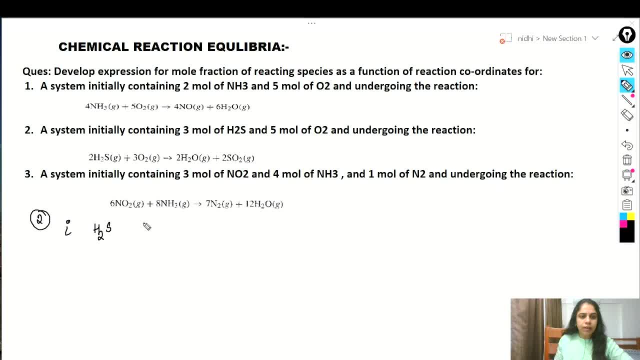 root over here component. so we have hydrogen sulfide oxygen water and soto, ok, and here we have mu soht means victorian and stoichiometric coefficient for the H2s is minus to, this is minus 3. these are the products, two and two, and this will be two to cancel and minus 1, fine. 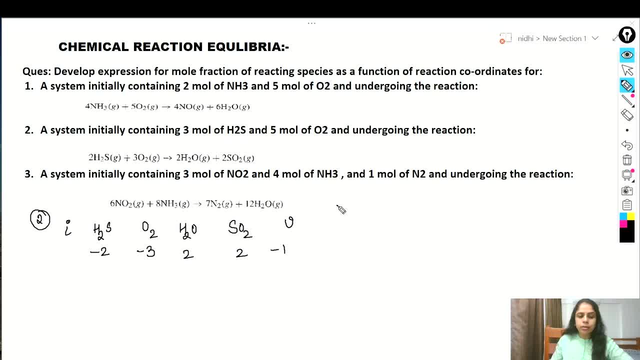 and initial number of total number of moles. so total contact number of moles. so total number of moles, moles for the second reaction, total number of moles which is equals to no. so here it is given 3 plus 5. so that will be equal to 3 plus 5, equal to 8. directly. we can write, we know the formula. so 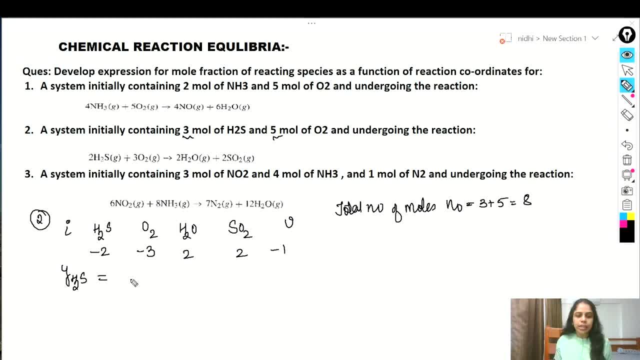 y. we just write down the expression yh2s. so initial number of moles for the hydrogen sulfide is given 3 mole, so 3 plus stoichiometric coefficient of hydrogen sulfide is minus 2 epsilon upon in the denominator. total number of moles are 8 and total stoichiometric coefficient 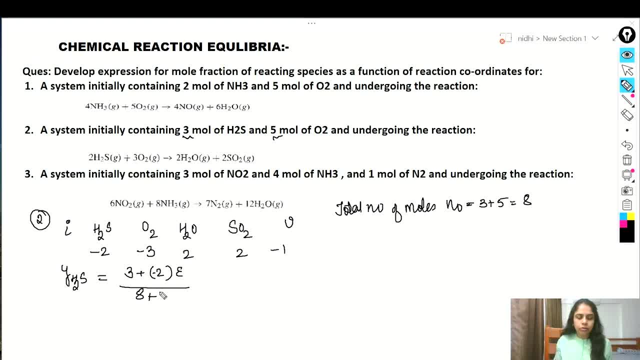 for the reaction is minus 1, so i'm just writing: okay, so let's write one more step, so that will be equal to 3 minus 2 epsilon upon 8 minus epsilon. now, similarly, you can write for the oxygen, so this will be equal to: 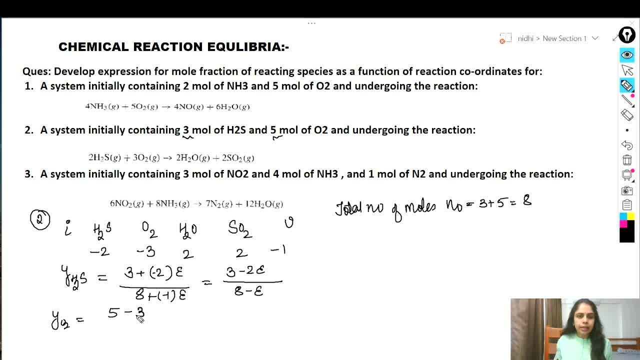 you, initial number of moles are 5 minus 3. stoichiometric coefficient minus 3 epsilon upon. and denominator is remain same for all the components. yh2o- this is equal to initial number of moles, for the h2o is none, so 0, that is not given- plus 2 epsilon. 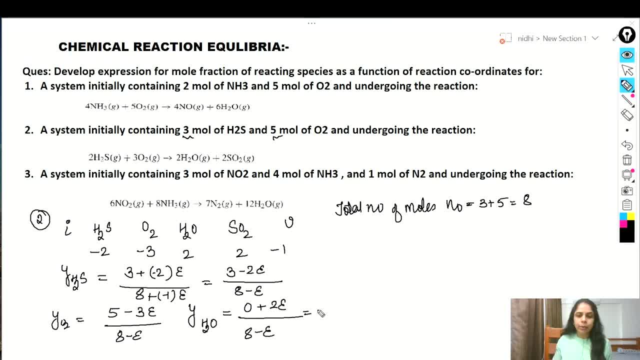 upon 8 minus epsilon, so that will be equal to 2. epsilon upon 8 minus epsilon. and the last�état, 2x2, is 8, so that will be equal to 2, and that is equal to 2x2 over 1, which. 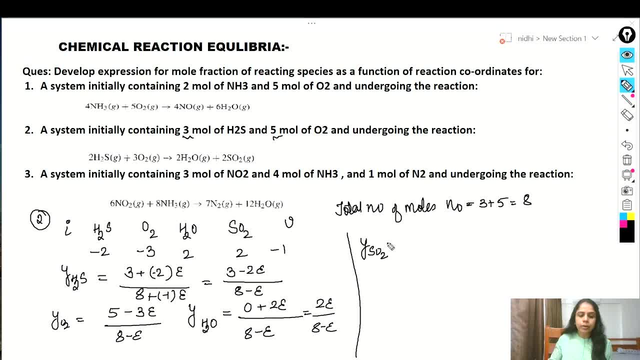 is equal to try to solve the two Personal alcohol equation so we can write the initial裆 defaults. last part of this is: ys2 is equals to 2 epsilon, because initial number of moles of SO2 also not given. so 2 epsilon upon 8 minus epsilon. so these are the four expressions for the second reaction. 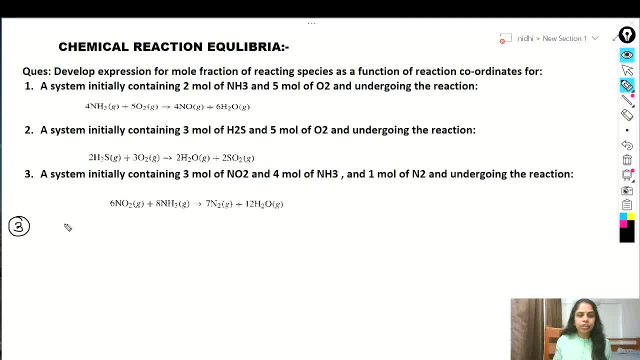 now let's discuss the last part, third part. so initial number of total number of moles, which is equals to NO, how much 3, 4 and 1. so 3, 4, 1 is 8. fine, now I'll just write down the species. so first is NO2, NH3, N2 and H2O. fine, and the stoichiometric coefficient is minus 6. 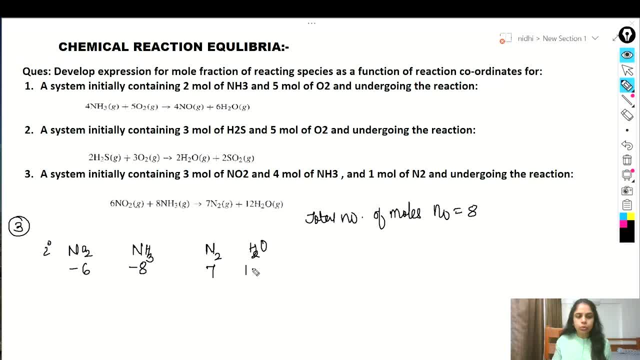 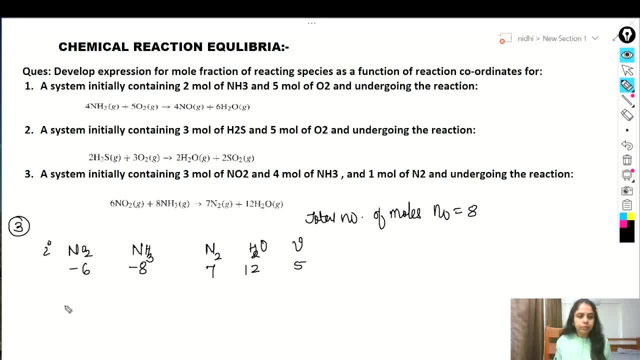 5. fine, and I'll just find out the mole fractions. so by NO2. so initial number of mole of NO2 is 3. stoichiometric coefficient is minus 6, epsilon upon in the denominator we have, total number of moles are 8 and overall a stoichiometric coefficient is 5. 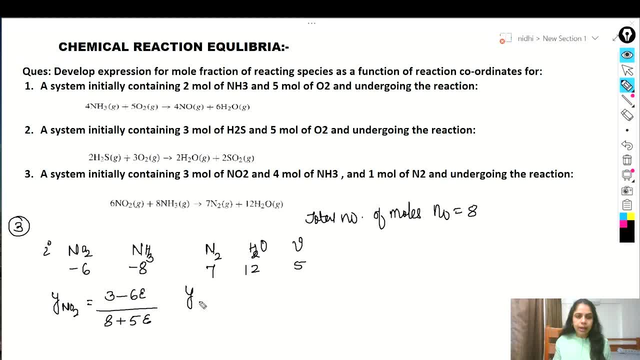 so this is the total number of moles of NO2, NH3, N2 and H2O, and H2O minus 8 and H2O minus 8 and H2O epsilon. so this is the first part. then by NH3, initial number of moles of of NH3 is 4. the 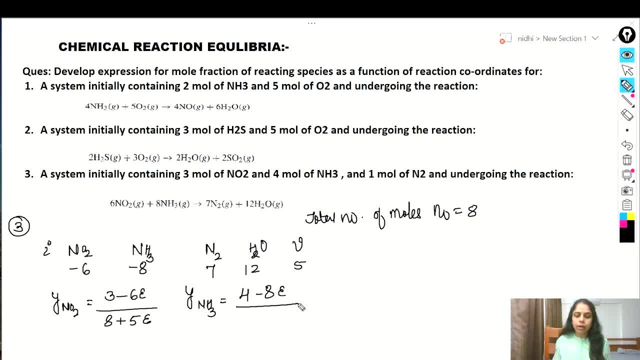 stoichiometric coefficient is minus 8 minus 8 epsilon upon denominator is remain same for all the components. and then we have YN2, which is initial number of moles of 1 plus 7 epsilon upon 8 plus 5 epsilon, and the last one is YN2. 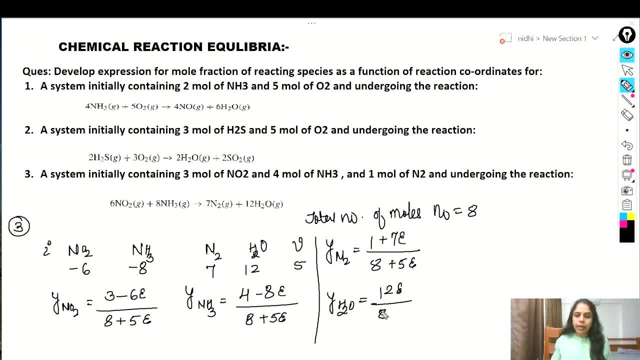 H2O, which is 12 epsilon upon 8 plus 5 epsilon. so these are the 4 expressions for the mole fraction of reacting species in terms of reaction coordinates. so hope you will be able to understand. these are the very simple and easy questions in our next video we will solve. 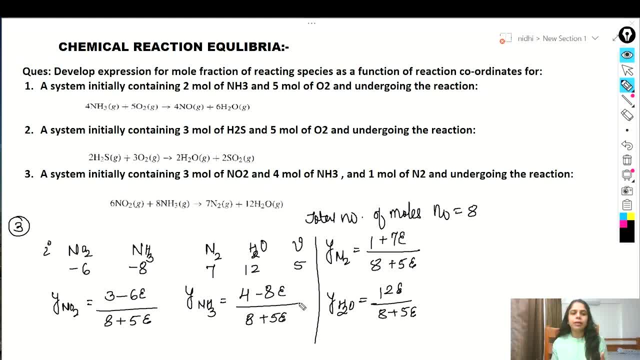 more. more questions related to reaction coordinates. thank you,